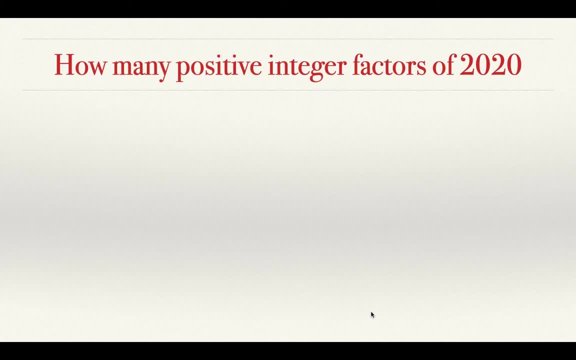 Positive integer factors of 2020 have more than three factors. As an example, suppose I am taking a natural number, 12.. Now we know that 12 has six factors, namely 1, 2,, 3,, 4, 6 and 12.. 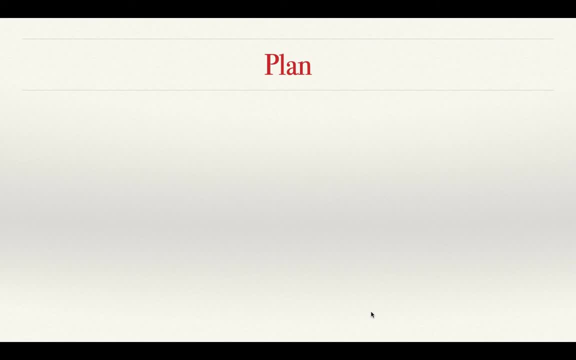 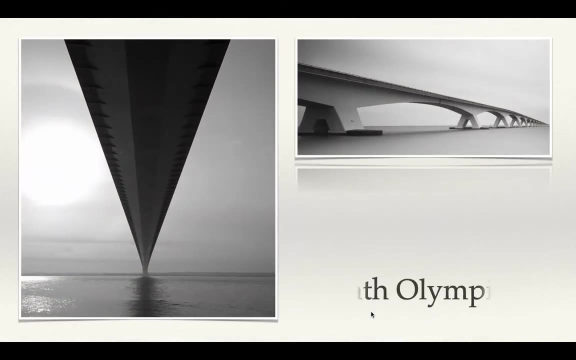 Before solving this problem, let's discuss a plan to solve this problem. First we will look for the concept, then we will try to find some hints and at the end we will discuss the solution. Now this type of problems are very important for math, olympiads and, at the same time, this problem. 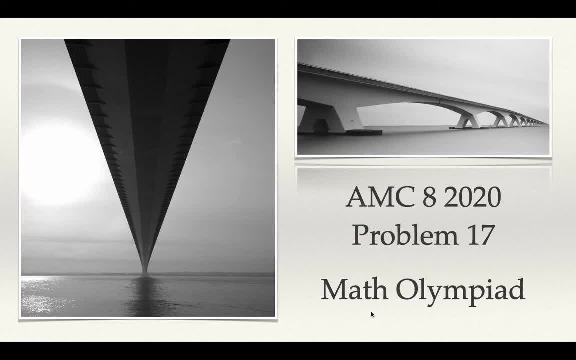 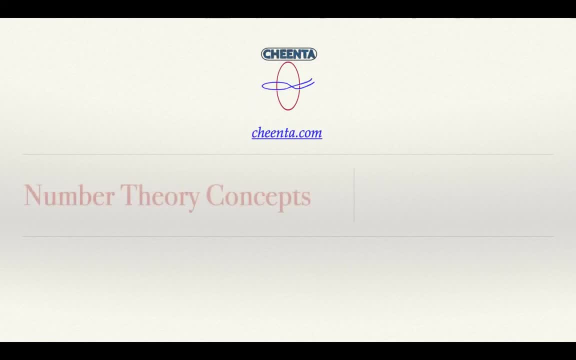 first appeared in AMCA 2020, problem number 17.. Hello everyone, this video is sponsored by cintacom. This video is based on number theory concept. Myself, shayantan Chakraborty, and I am a content creator at cinta. Now let's look for the concept. 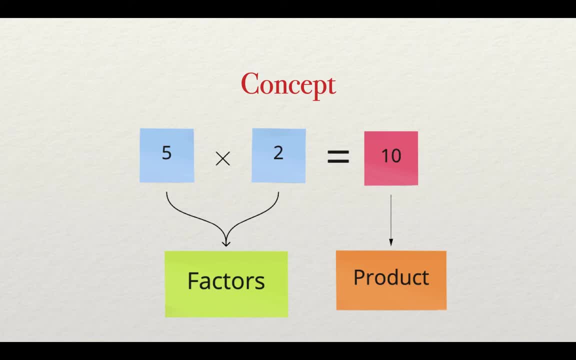 When we are dealing with factors, first we have to know the basics. Suppose I am multiplying 5 and 2 and I am getting a result as 10.. So 10 here is the product and 5 and 2 are the factors of 10.. 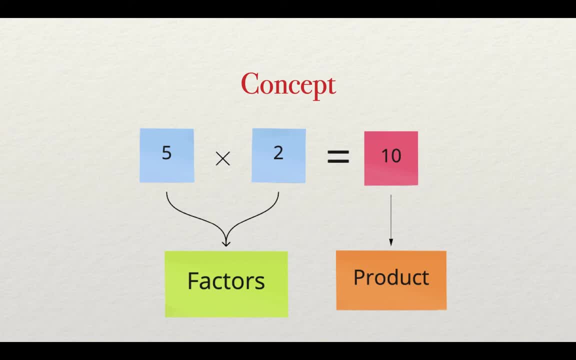 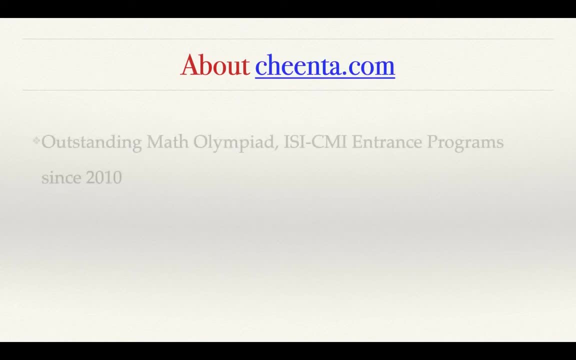 As we are calling them factors. It means 10 will be divisible by both 5 and 2.. A little bit about cintacom. Cinta is running since 2010 with brilliant students in mathematics. Cinta trains their students for several math olympiad. 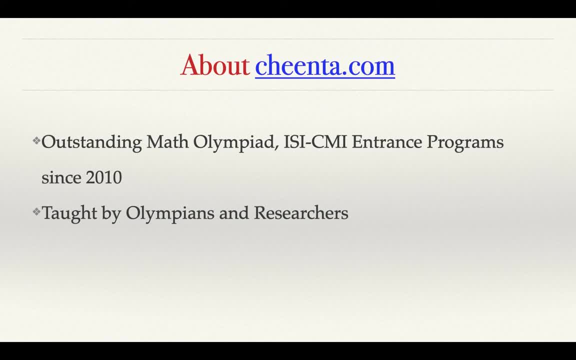 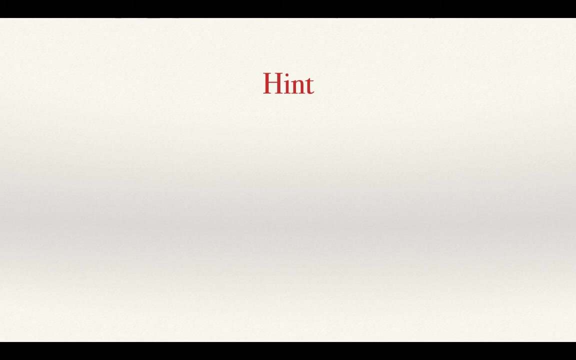 isi, cmi entrance programs which are taught by olympians and researchers at cinta. We also have a free toolbox Where we post several problems for everyone. Please do check it out. The link is given in the description. Let's look at the first hint: List: all positive integer factors of 2020.. 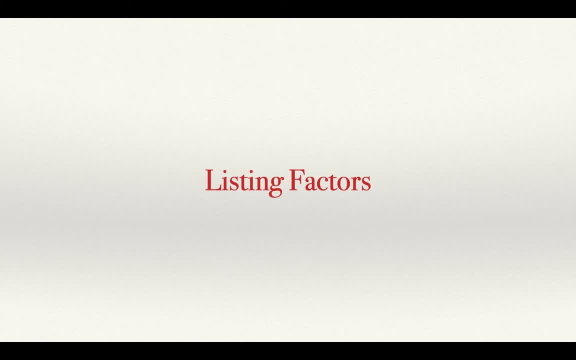 Our first step of solving this problem is the listing of factors. Now, before doing that, Let's check one example calculation. Suppose we are asked to find all positive integer factors of 1024.. We can do this very easily. Now for our problem. 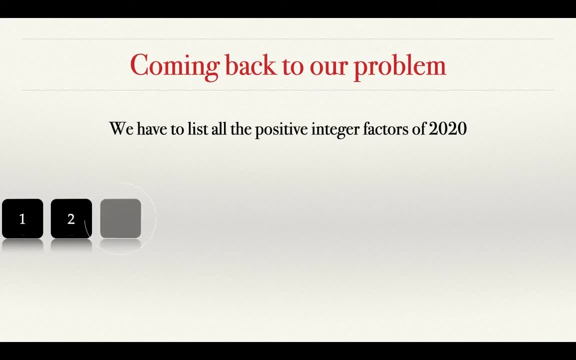 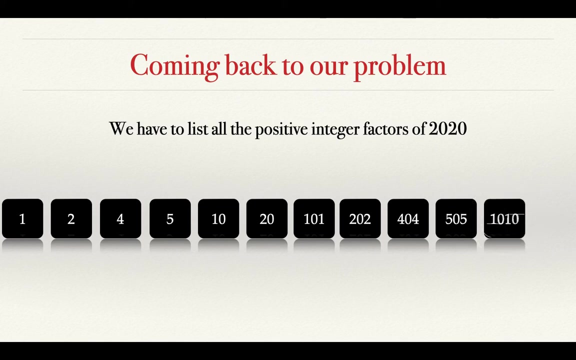 We can do it by the same way. The factors will be 1,, 2,, 4,, 5,, 10,, 20,, 101,, 202,, 404,, 505,, 1010, and 2020 itself. 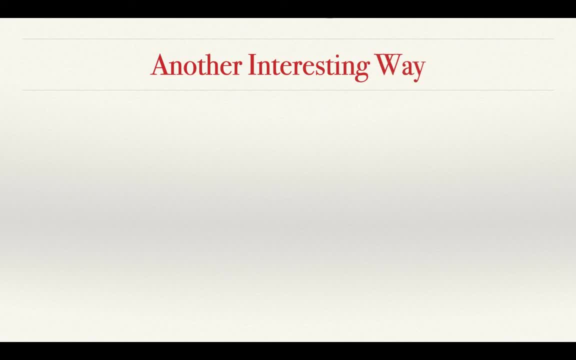 Another interesting way, as the previous way can be very time consuming for larger numbers. So first let's look at the definition. The number of positive divisors of a positive integer n is denoted by tau n. If the canonical form of a positive integer n greater than 1 be n equals p1 to the power alpha 1,. 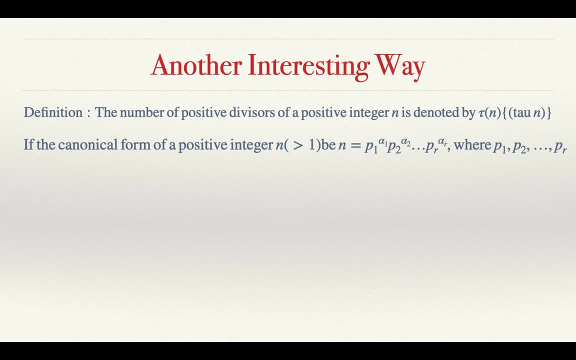 p2 to the power, alpha 2 up to pr to the power alpha r, p1 to pr are distinct. prime and the exponents alpha i are all positive. Then tau of n equals alpha 1 plus 1 multiplied by alpha 2 plus 1 up to multiplied by alpha r plus 1.. 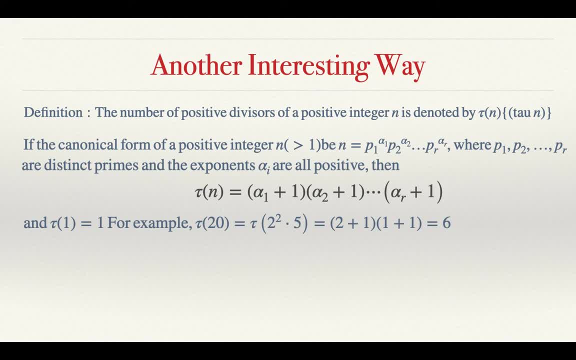 We must remember that tau of 1 is 1.. Now this definition and the canonical forms looks very much complex at first sight, but it is very easy when we look at an example. Suppose I am taking n equals 20.. Now our first step will be the prime factorization of 20, which 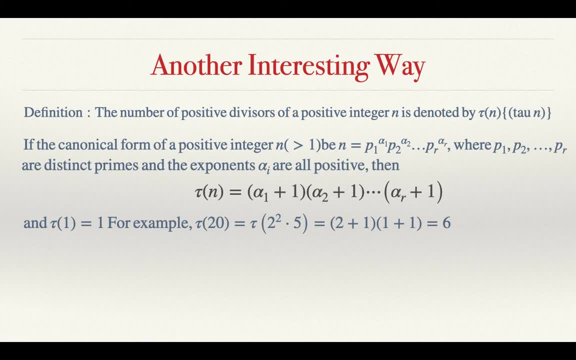 is 2 squared times 5.. Now for 2 squared, we have to take the power and add 1 with it. So for 2 squared we have 2 plus 1, and for 5 the power is 1, so we have 1 plus 1.. So we have 3 times 2, which. 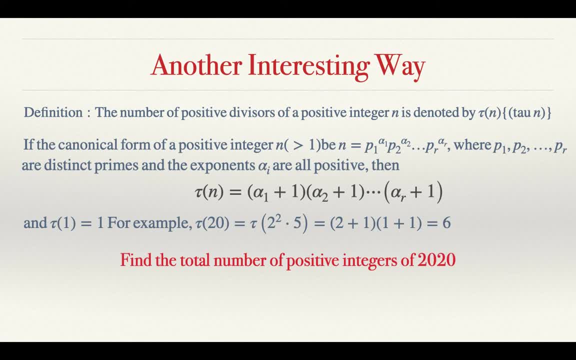 is 6.. Now let's apply this process for our problem for 2020.. The prime factorization of 2020 is 2 squared times 5 times 101.. Now tau of 2020. first we have to find the prime factorization. 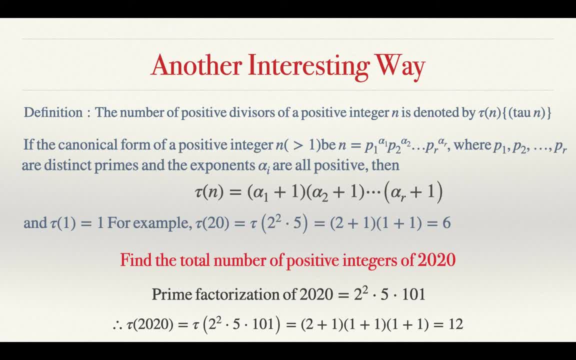 which we have already found, which is 2 squared times 5 times 101.. So for 2 squared, we have 2 plus 1, for 5 it is 1 plus 1, and for 101 it is 1 plus 1.. So multiplying these three, we are getting. 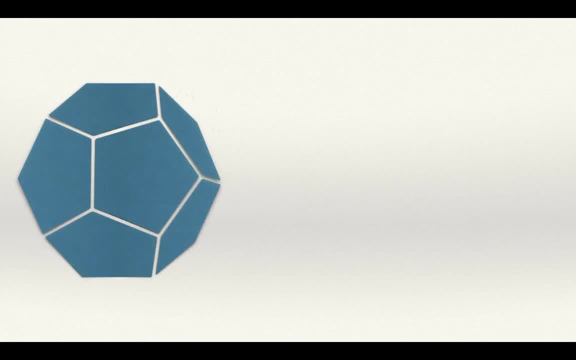 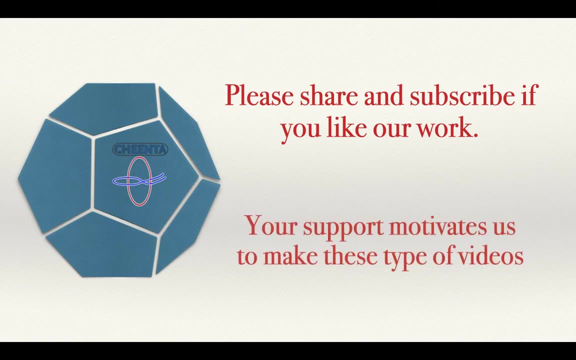 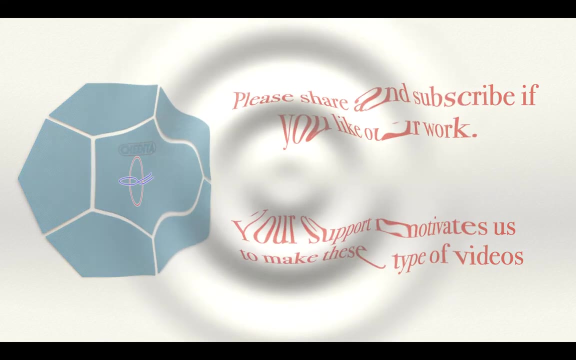 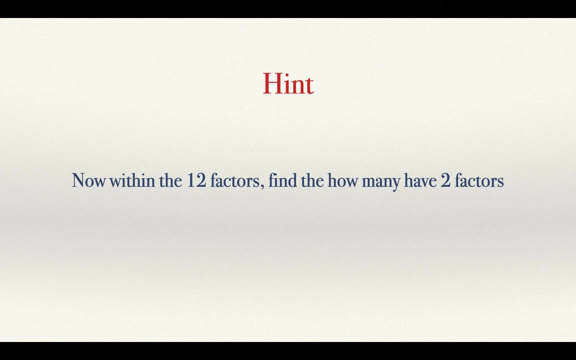 12. A big shout out to all of you guys who have shared and subscribed our work. Please do share, like and subscribe more so we can make more content like this to motivate several people. Now let's look at the next hint Now. within the 12 factors, find how many have two factors. 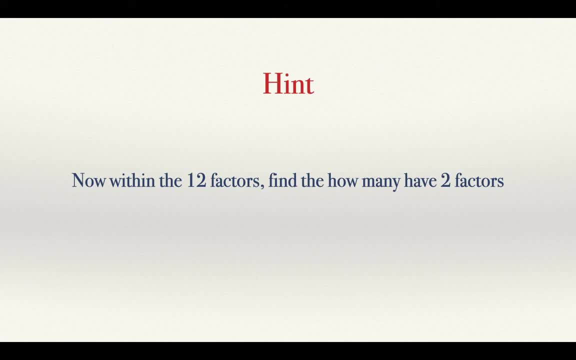 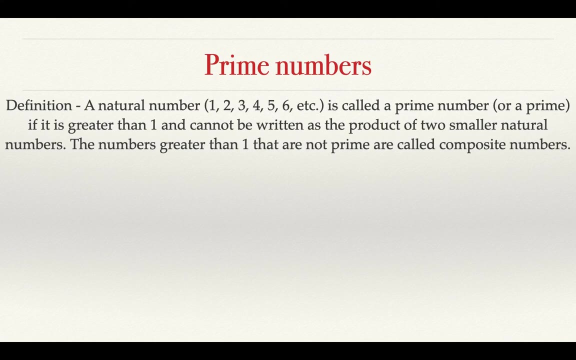 It means from the factors 1 to 2. Of 2020, how many have two factors? Before doing that, let's check the basics. Prime numbers: A natural number- 1, 2, 3, 4, 5, 6, etc. is. 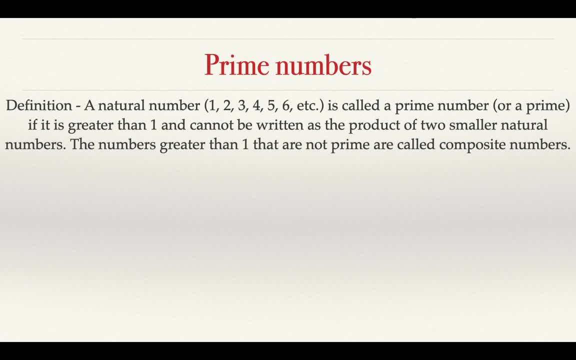 called a prime number or a prime if it is greater than 1 and cannot be written as a product of two smaller natural numbers. The numbers greater than 1 are not prime, they are called composite. One interesting fact: that 2 is the smallest prime and the even prime, and it is unique, I mean there. 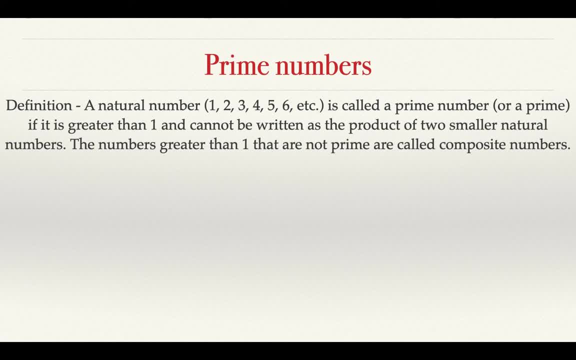 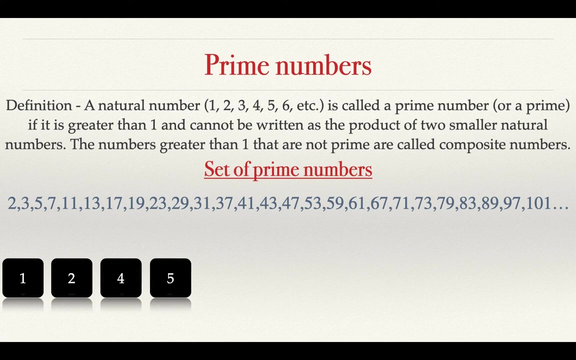 is only one even prime, and that is 2.. What are the set of prime numbers? This is basically the set of prime numbers from 2 to 101.. Now we will will list the positive integer factors of 2020, because we have to find the. 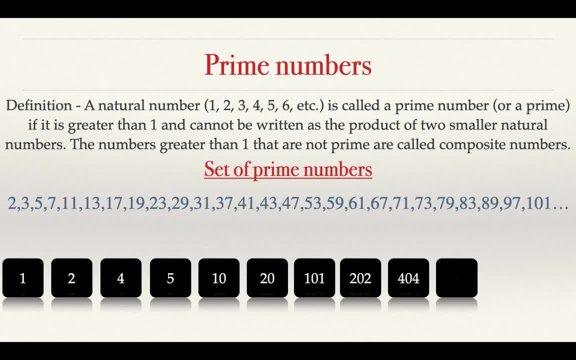 number of prime numbers in the factors of 2020, as they have two factors. these are the factors of 2020. 2501 is present in the factors of 2020, hence 25 and 101 are prime and they have two factors, so they won't be in our set. now let's look.